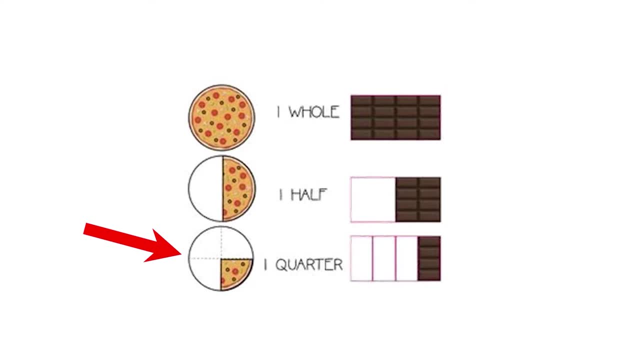 Whole, half and quarter. We can have it in a circular shape or a rectangle. So, for instance, you can see the pizza, a whole pizza, a half of the pizza and a quarter of the pizza. Then you can see a bar of chocolate. 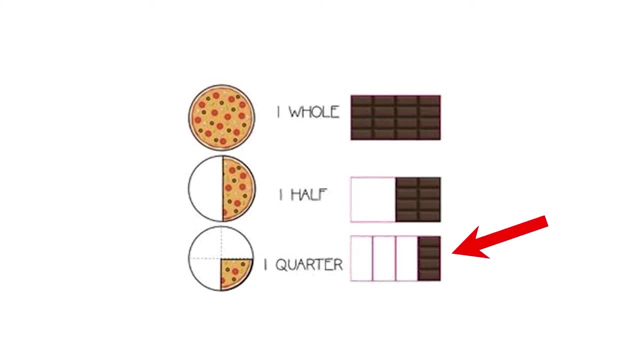 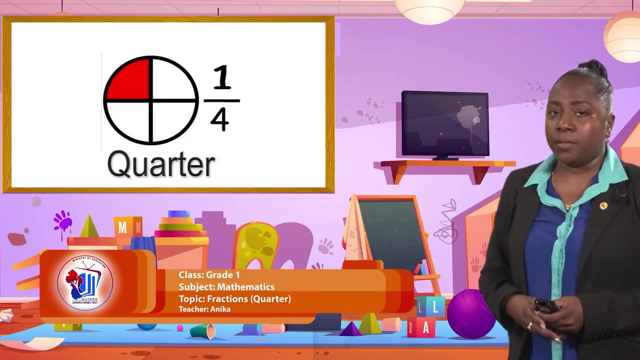 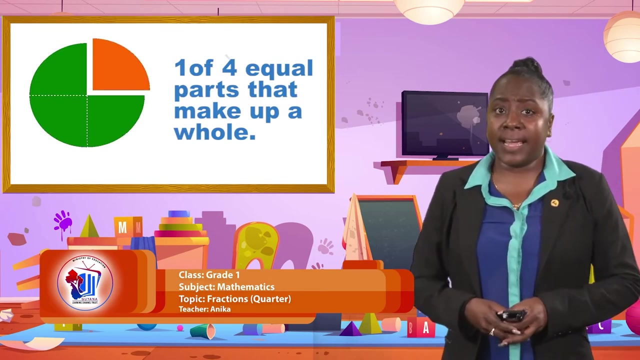 a half of that bar and a quarter Quarter is simply one out of four parts, And this is how it's written: The number one at the top and four at the bottom. If you look at the circle that I have on the screen, it's divided into four equal parts. Remember when we're doing fraction. 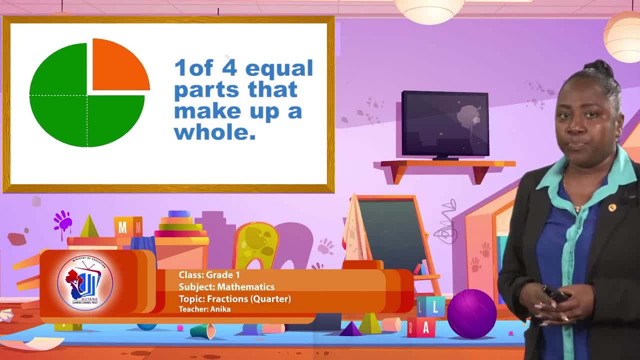 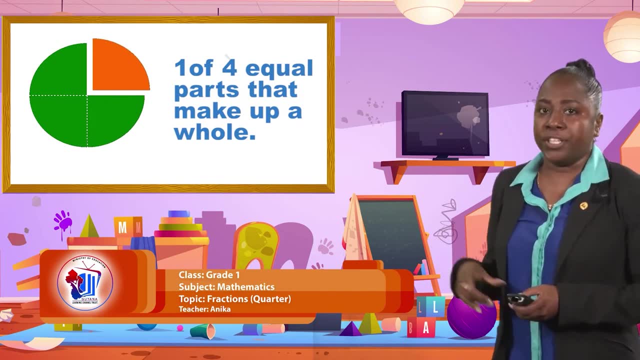 the parts. they need to be divided equally. Three parts are shaded in green and one part is shaded in orange, One of four equal parts that make up a whole. So we have the orange, which is one out of the four parts that makes up the whole circle. 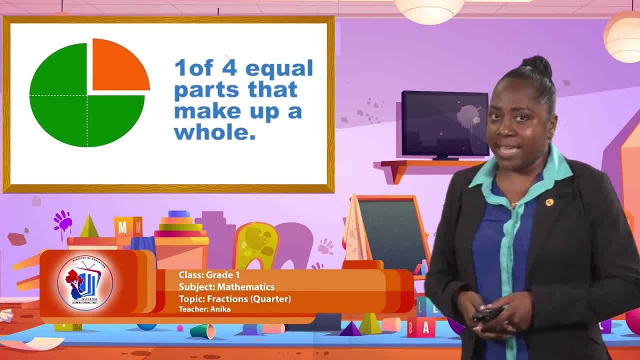 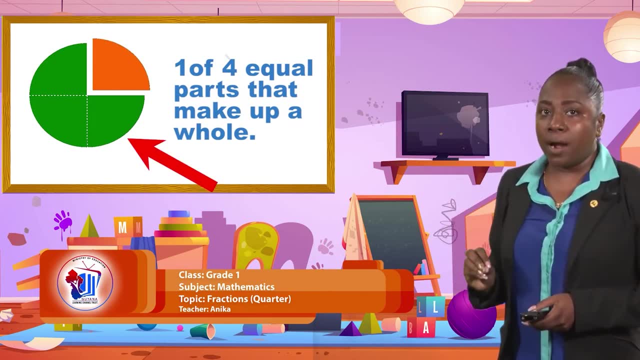 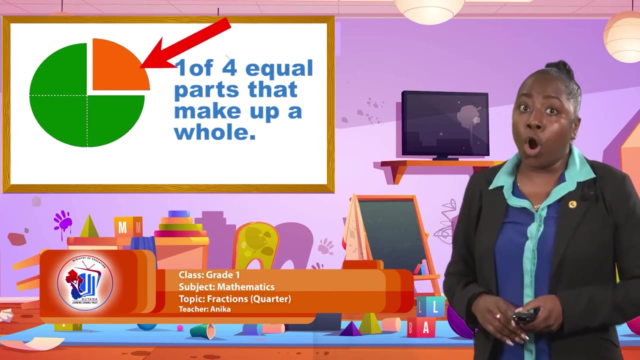 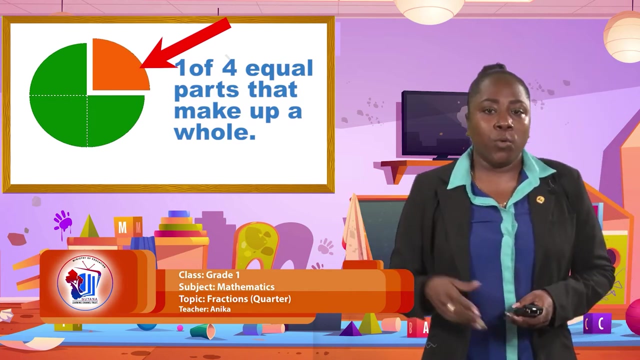 Understood. Let me explain it again. We have a whole circle and it's divided into four equal parts. Three parts are shaded in the color green. Then we have one part that is shaded in the color orange. That one part represents a quarter, One quarter which is one of four equal parts. 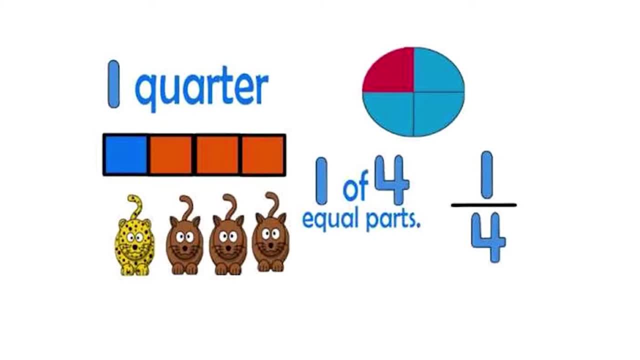 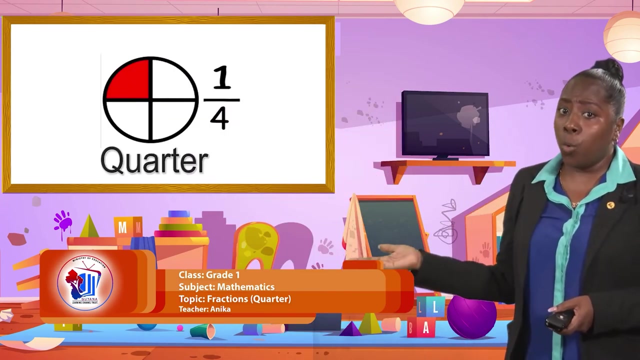 Look at the examples on the screen. We have a rectangle divided into four equal parts. We have discernment Circle divided into four equal parts And we have a group of cats. We can divide them into quarter. Let me see if you understood what I said. Remember, this is the way we write a quarter. 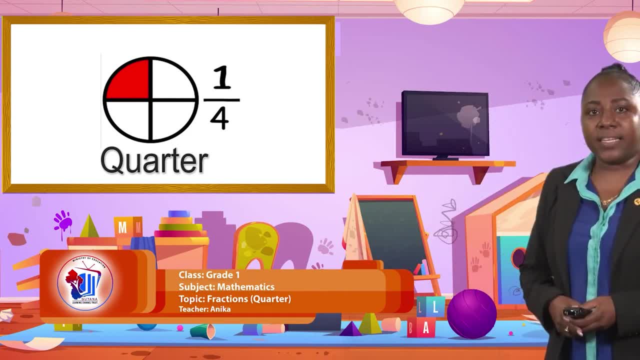 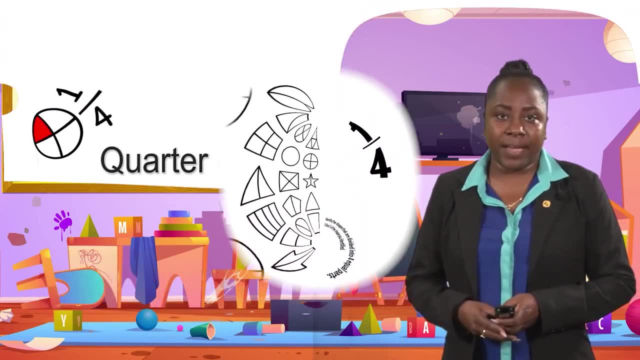 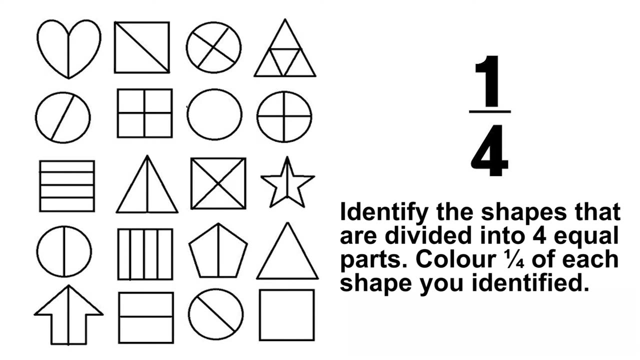 We are going to identify the shapes that are divided into four equal parts. After that, we are going to color quarter of the shape you identified. So take your time, Look at the shapes that are displayed. Remember when we are speaking about quarter. 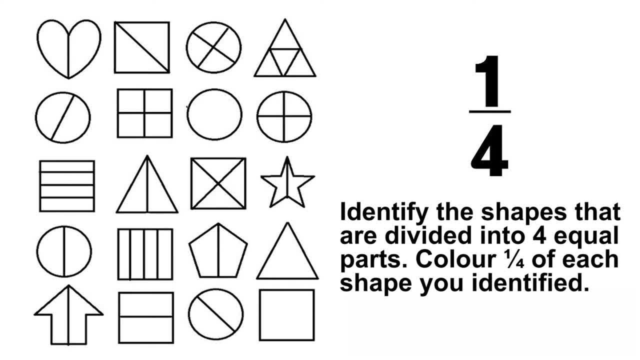 we are speaking of one of four parts, Meaning the shape has to be divided into four equal parts, And you are going to see which one we can shade to identify a quarter. So take your time. We have many shapes on the screen. Go through them and when you find one, that is divided, 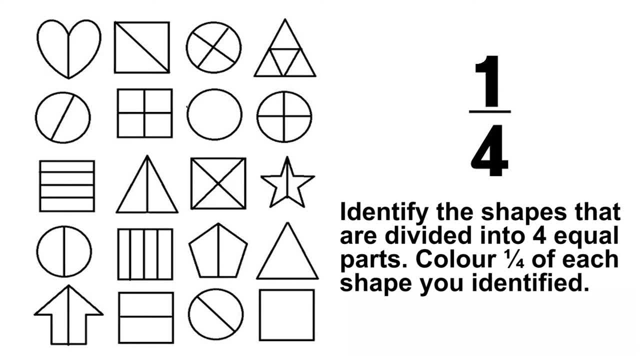 into quarters. you are going to color one part, meaning you are going to identify a quarter of that shape. So take your time, Go through them, See which shape you are going to identify, Follow the instructions and then we're going to check on your answer. 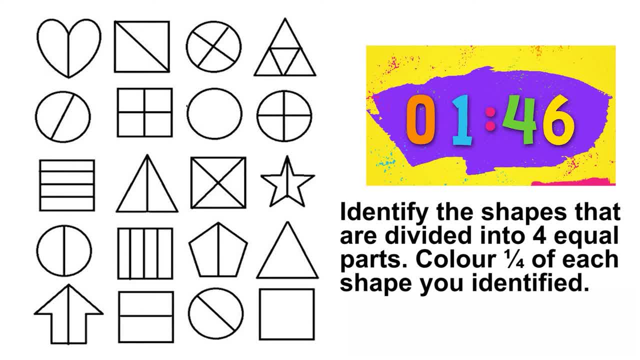 So it looks like we have two, four, So the first one is a quarter. In this example, you are going to find a quarter of what it would be, So we are going to take a quarter as well. So the first one is a quarter. 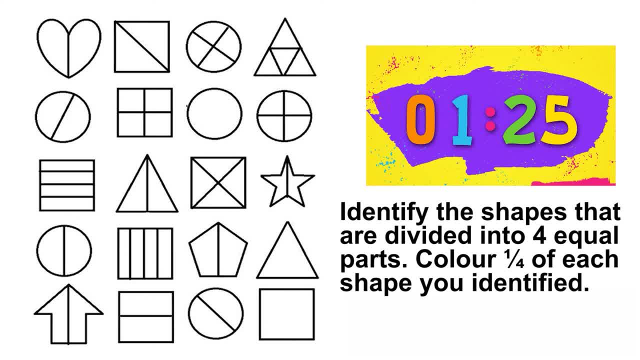 In this example, you are going to find a quarter, So we are going to take a quarter of the shape. We'll be right back. We'll be right back. We'll be right back. Completed. Let's look at the first part. 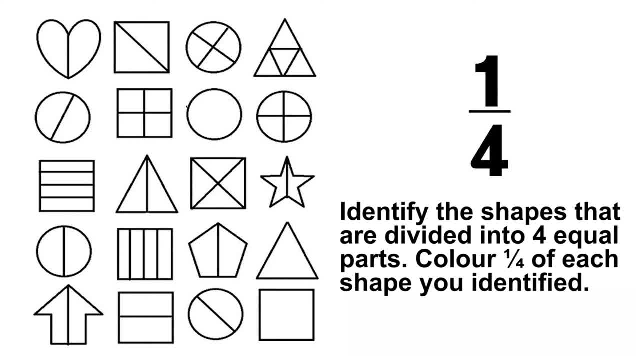 We had to identify which shapes are divided into quarters or four parts, And that was very easy to do. We have the circle, the triangle, the square on the second line, the circle on the second line. Then we have a square on the third line. 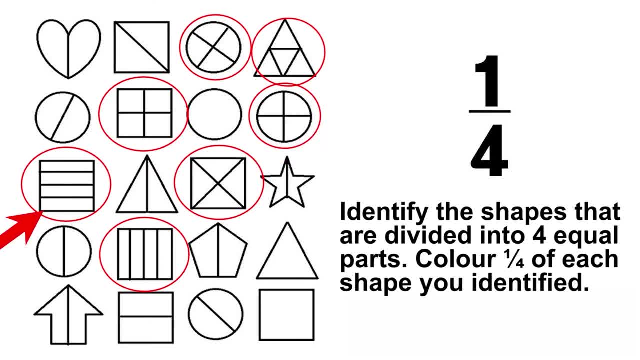 You can see two. One has an X, One has some horizontal lines. Then, in the fourth line again, you can see another square divided into four equal parts. Very easy, We have more shapes there, but some are whole and some are divided into halves. 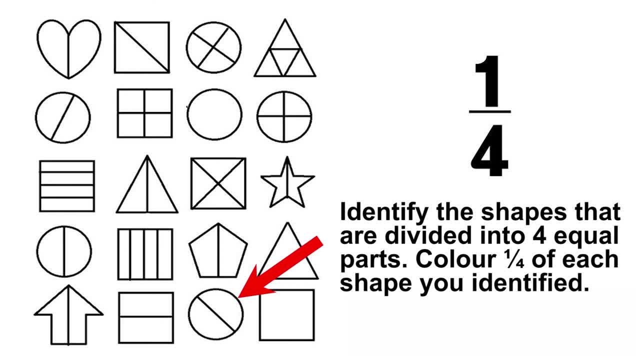 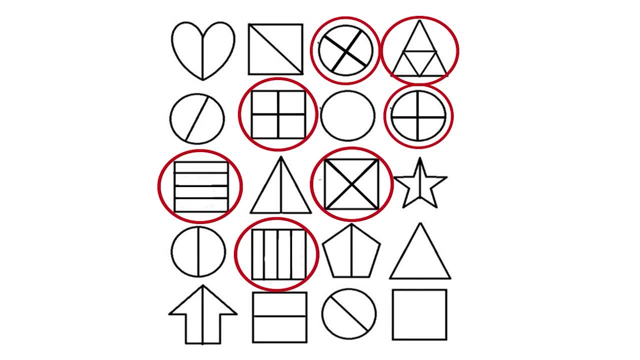 That's not what we wanted. We only wanted the ones that are divided into four equal parts. So check your answer, See if you're having these correct, And then we're going to go to the next part that I asked you to do. 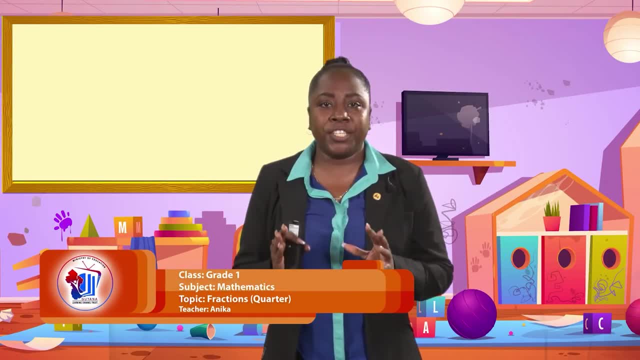 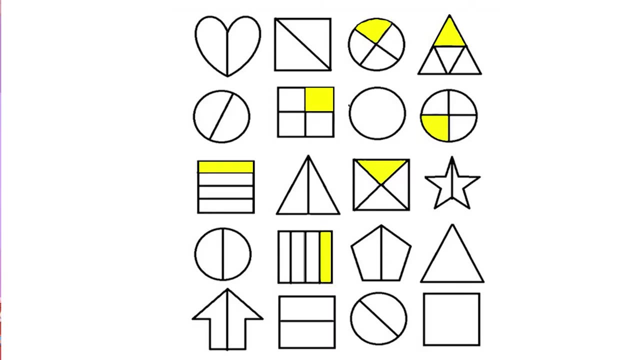 I also asked you to color quarter, meaning one of the four parts of the shapes that you would have identified. Check on the screen and see if that's what you did: Shaded one of the four parts. If you did, then it's correct. 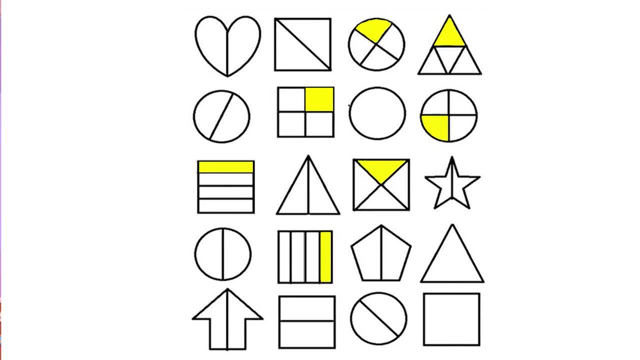 If not, I still applaud your effort for trying Not to worry. You're going to get it. Simply look for all the shapes that are divided into four equal parts, and you are only coloring or shading One part. You could have used your crayon. 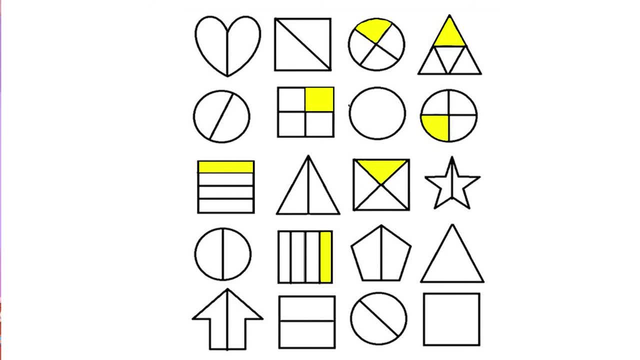 or your pencil Doesn't matter. Point is, I want you to shade only one part. So if you shaded two parts, that means you shaded half of the shape. And we're not looking at halves today, We're looking at quarter. 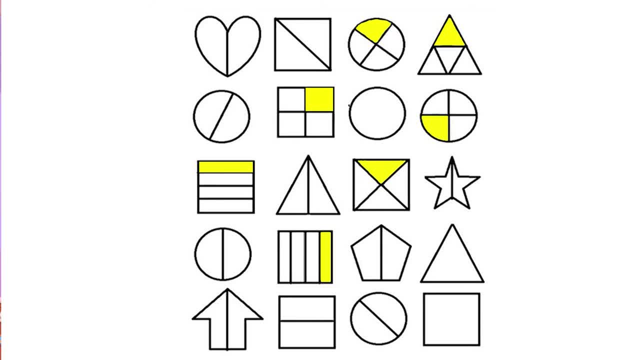 So look on the screen, go through them one at a time and see if you did the exact same thing. If you didn't, then I'll advise you to maybe draw the shape and shade it inside of your book. Remember, we're looking at quarter. 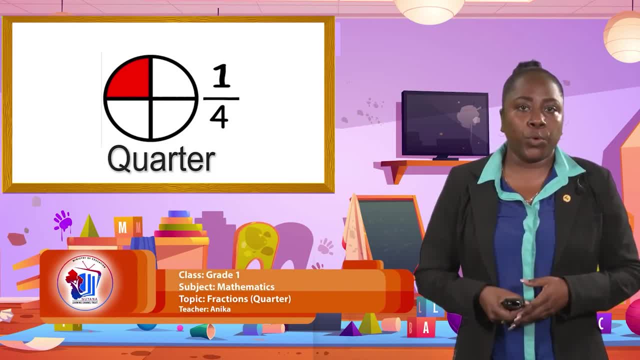 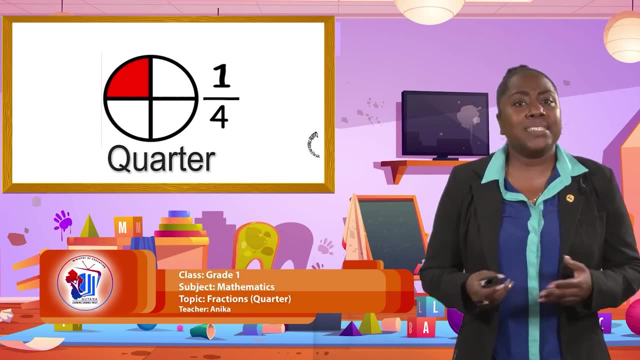 Let's spell the word quarter Q-u-a-r-c-e-r quarter. A quarter simply means one of four parts, But not just four parts: four equal parts. Sometimes, when we share things, we like to take the biggest part or portion.